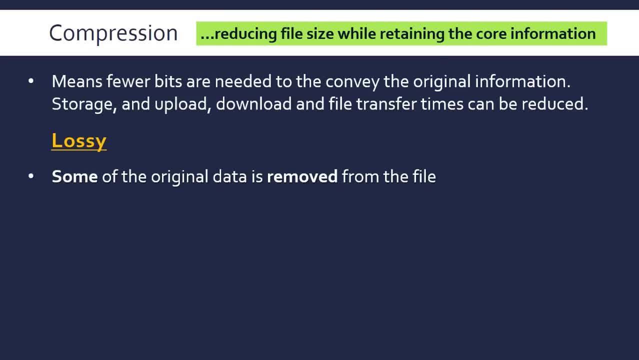 And this is where the algorithm actually physically removes data from the file. So clearly, the file size gets reduced and it's quite effective, but some data is lost when you apply this compression, So this wouldn't be used where all the data in a file is important. 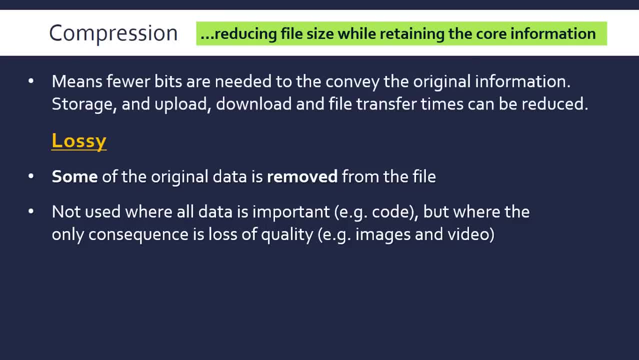 For example, with any text like source code. you can't afford to just chop off bits of a text document, for example, But you may want to apply this where the only consequence really is a loss of quality. So, for example, with images and video. 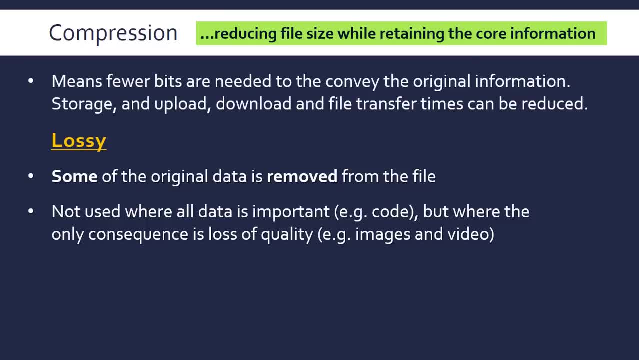 they can have very, very large file sizes if the quality is amazing. but you can maybe sacrifice some quality if it saves you a lot of time and storage space. So a consequence of lossy compression is when you or if you can decompress it afterwards, the file isn't the same as the original. 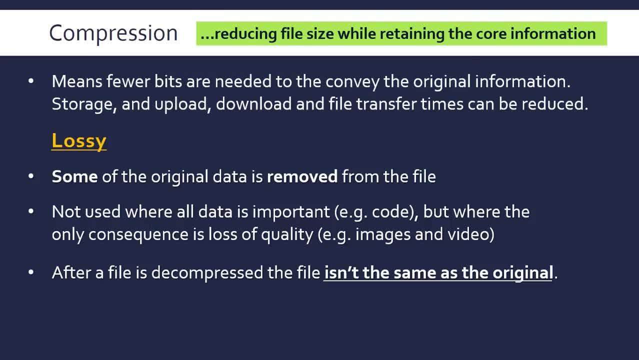 So obviously in some cases where you perhaps export an image from Photoshop and put it into a lossy format, you're not going to have a chance to decompress it, because the image is an image. But if you had like a zip file in Windows where you compress it and then decompress it after, 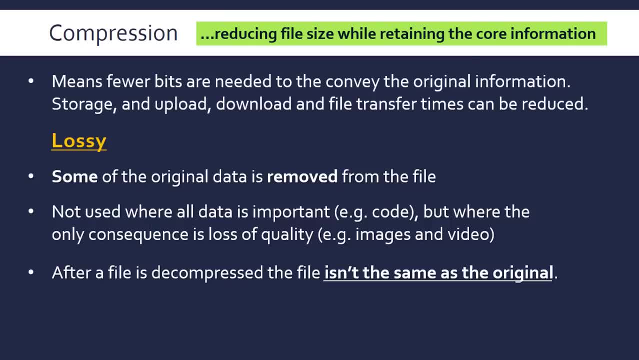 it wouldn't be the same as the original if lossy compression was used. So two examples of lossy algorithms are JPEG for images and MP3 for audio, and they're quite complicated in terms of their operation. But one of the things they can do is remove background noise or just pictures outside our human range or colours we least recognise. 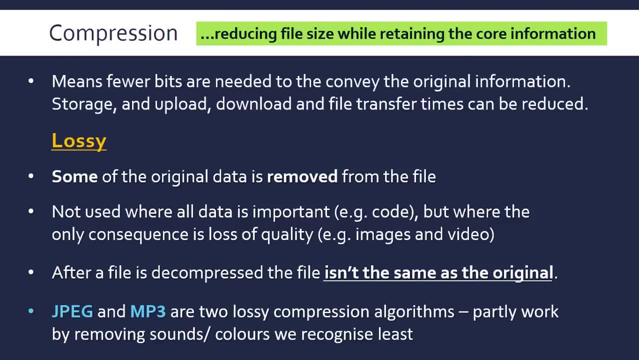 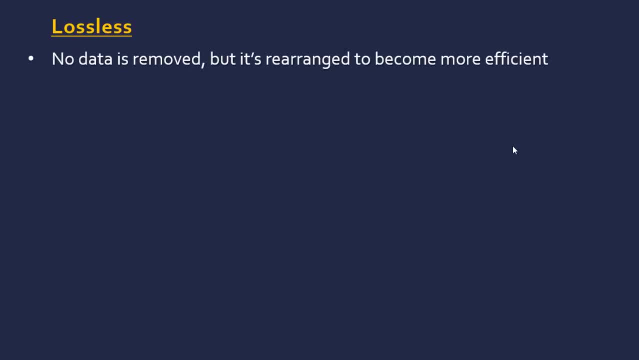 So basically removing data that, as humans, we're least likely to recognise or notice as gone. In contrast to lossy compression, you have lossless compression which, as you'd expect, doesn't actually delete any data from the file, but it's rearranged the data to make it more efficient to where it can. 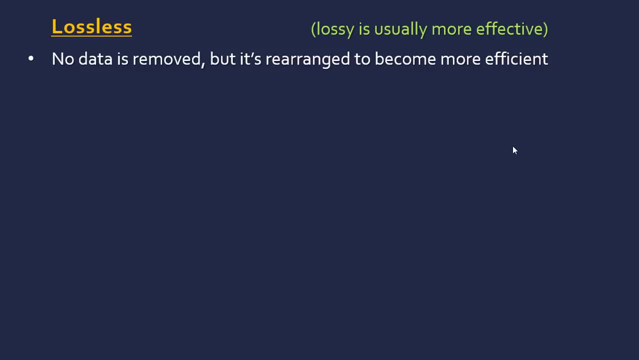 So lossy is usually more effective than lossless, but clearly lossless is important where you don't want to actually delete any of your data. All of it's important, basically. So one way this can be done is with run length encoding RLE. 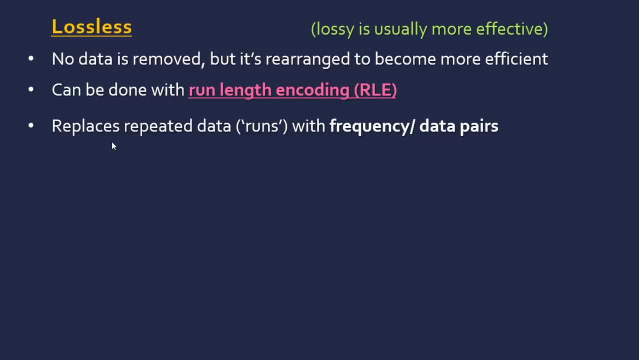 This is all about kind of compacting repeated data. So repeated data or kind of consecutive data is called a run, And so we replace long runs with frequency data pairs. So the best way to show this is with an example. So an image is a common. 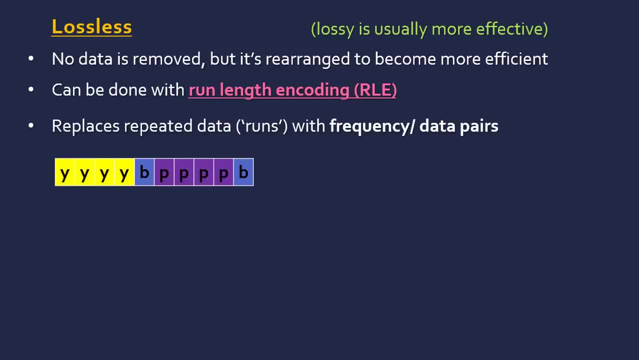 Where it's a common place, this might be used. So you have blocks of colours in an image. So you've got four yellow, you've got blue and four purple, then another blue, And you could replace this with these pairs of frequency: first, and then the data.